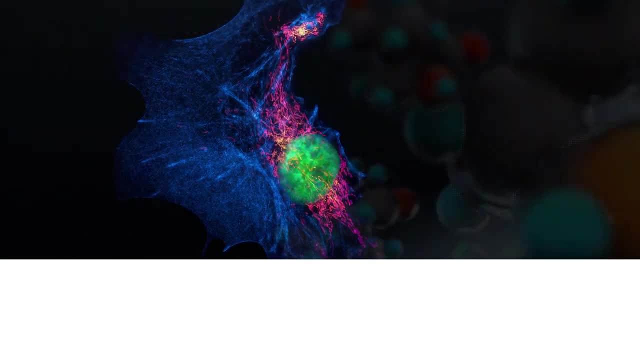 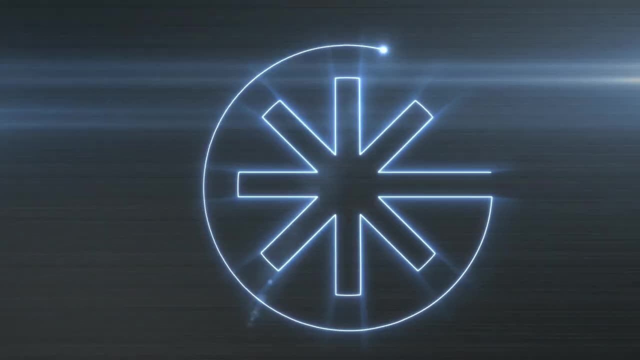 First, we are going to make a simple, easy-to-use and easy-to-use paper flower. First, we are going to make a simple, easy-to-use and easy-to-use paper flower. First, we are going to make a simple, easy-to-use and easy-to-use paper flower. 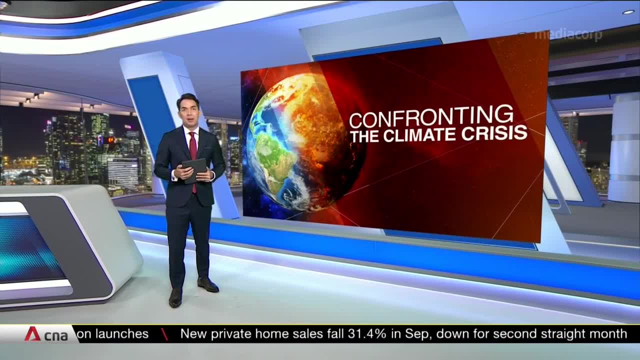 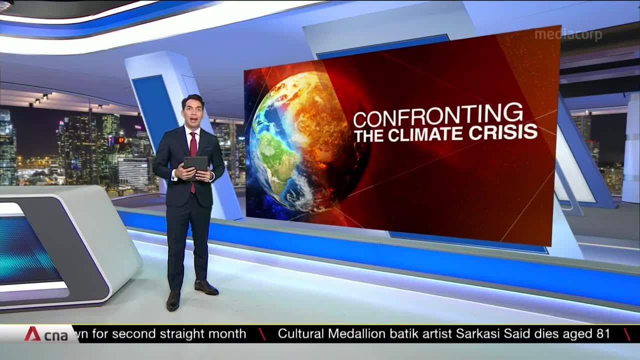 Discussions at the UN Climate Change Summit at the end of this month will center around cutting greenhouse gas emissions, but they'll also touch on adaptation. Lo Kwe Su reports on how we will need to figure out ways to live and survive on our changing planet. 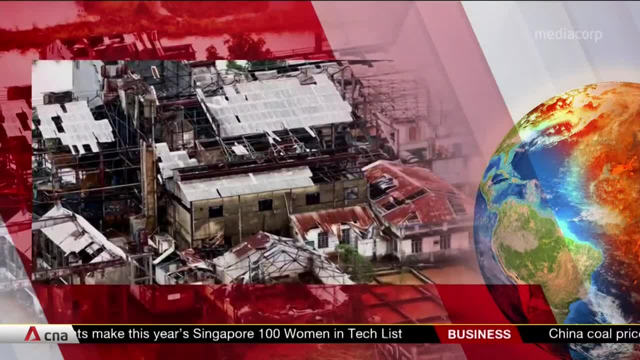 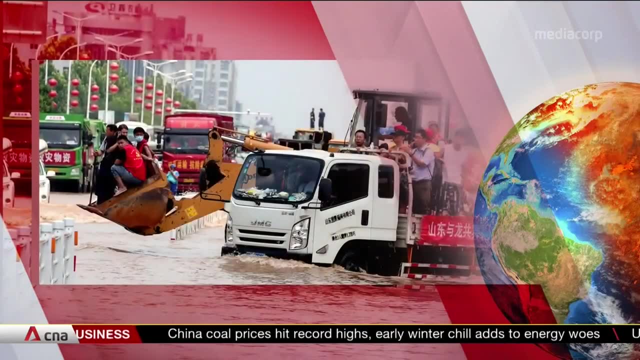 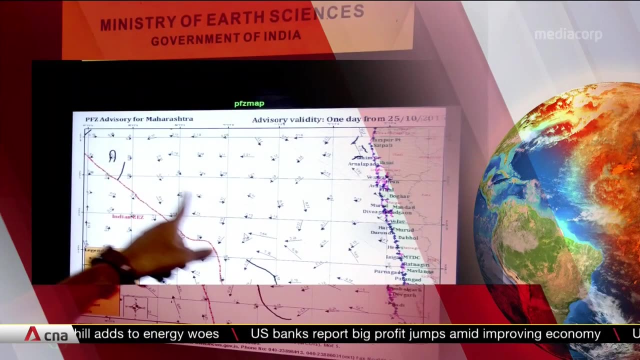 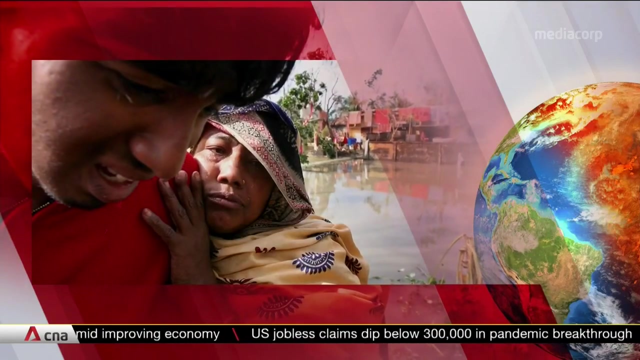 Changing what we grow and how we grow it. Rethinking how we store, make and transport what we need to keep our economies running. Ramping up our defences so we can react in time And when even these are not enough to keep us safe, relocating entire communities so they can start life elsewhere. 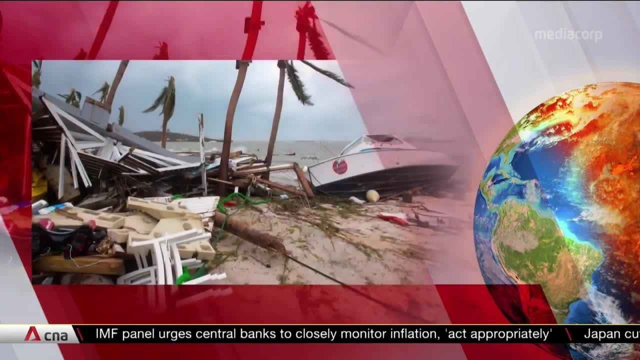 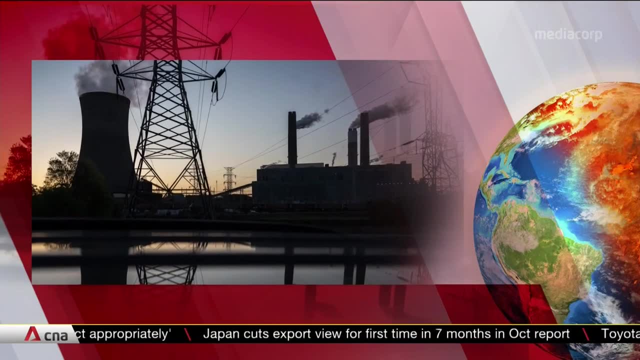 Just some of the hard choices we have to make to cope with a climate that has changed, that is still changing and that will continue to change whatever we do or fail to, And what we need to do to mitigate the emission of gases driving this change. 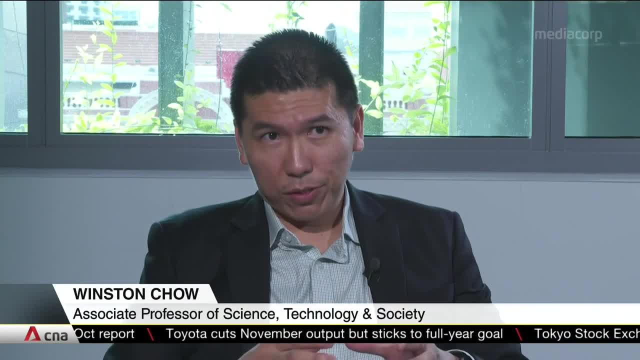 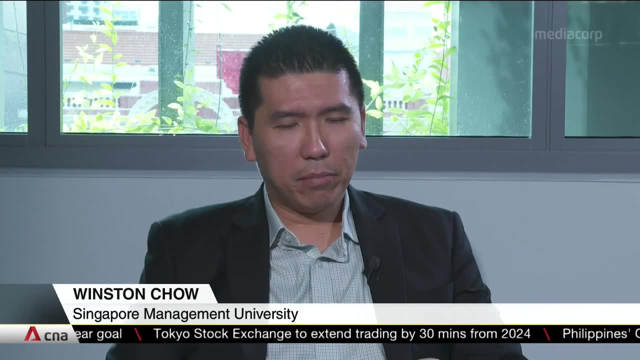 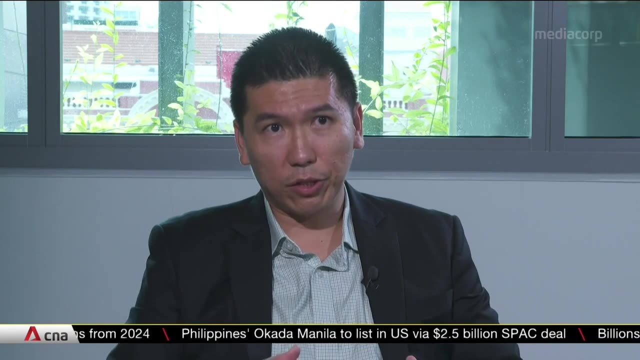 Mitigation is the process of attacking the causes of climate change. You want to reduce your carbon dioxide emissions. you want to reduce deforestation, But mitigation by itself will not stop the worst excesses of climate change from affecting society in general. Therefore, you need adaptation. 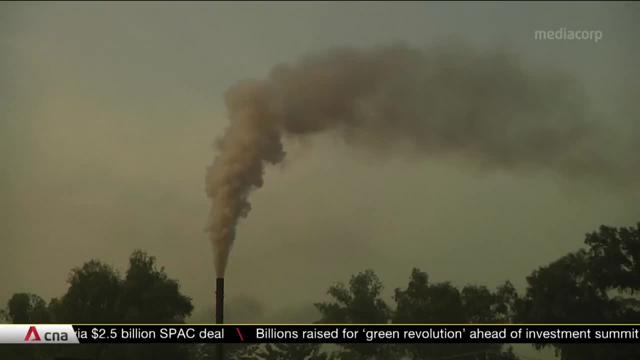